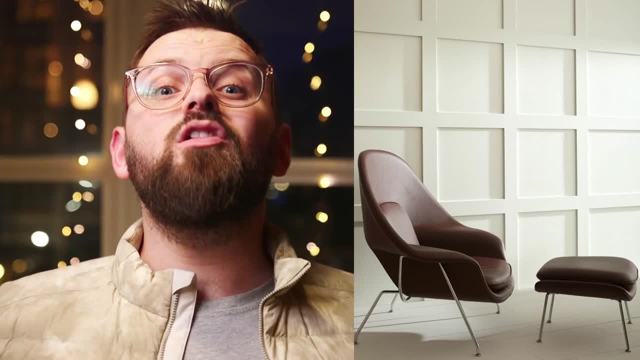 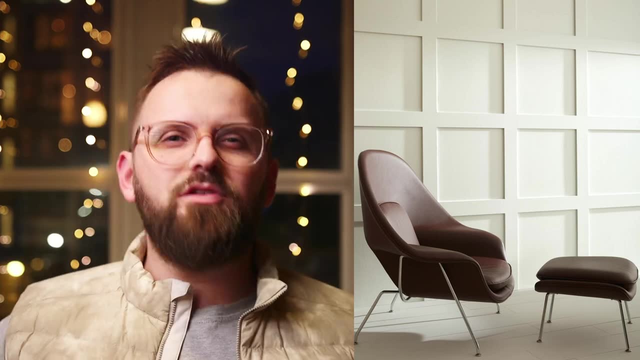 neutral it ends up feeling. I've used Oxford White all over a house for that reason alone- Like everything inside. So a color like that really allows Edge Comb Gray's subtle undertones to be featured, because it's not trying to compete with it, And I think that's very important in this case. 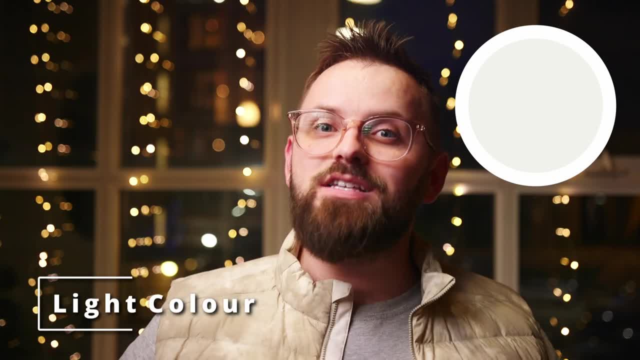 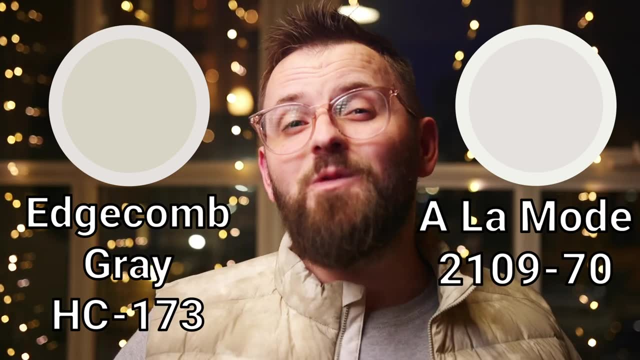 Next we're going from white to light, And that color is A La Mode. This is a color from the Color Preview Collection by Benjamin Moore and it's notated by the color code 2109-70.. Sometimes, when I have a light color pairing for an already fairly light color like Edge Comb Gray, 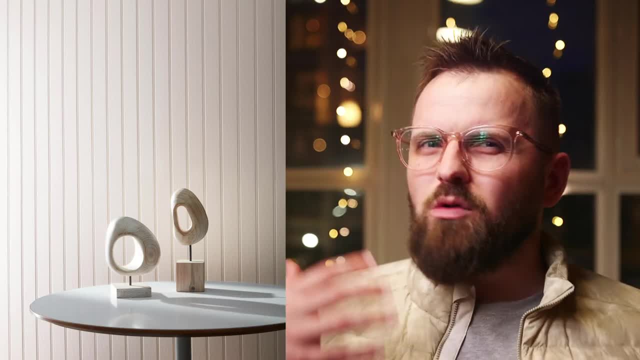 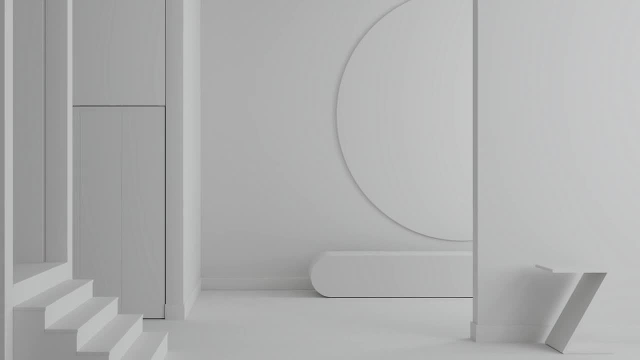 I sometimes go with something similar. You can kind of pick one or the other, But A La Mode was selected to be used in conjunction with Edge Comb Gray. Not only is it quite a bit lighter as a color, it also moves away from that kind of 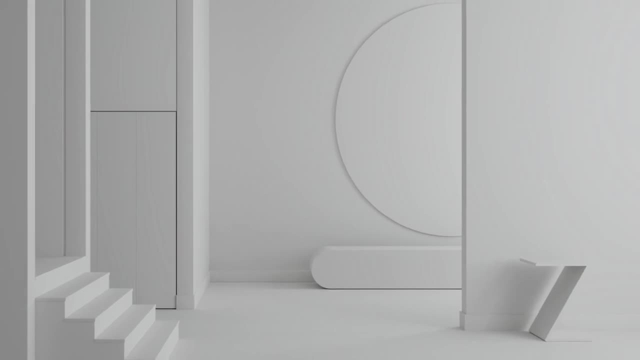 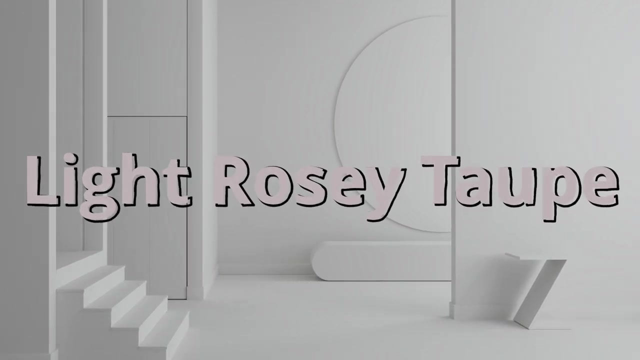 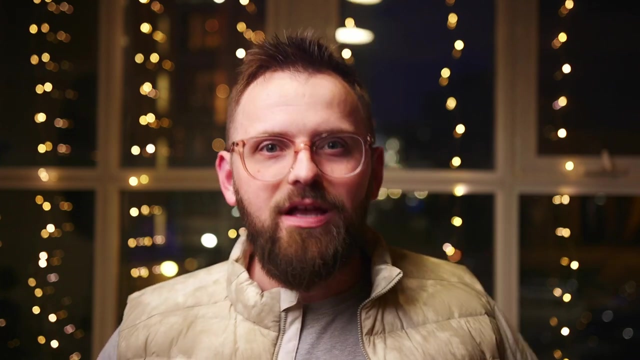 grayish, yellowy, warm side of Edge Comb Gray to an almost light rosy taupe where A La Mode has tiny bits of pinky, brown and gray. You can really feel that polarization when you have it next to Edge Comb Gray, because even though they're both pretty subtle, you start to see how each color 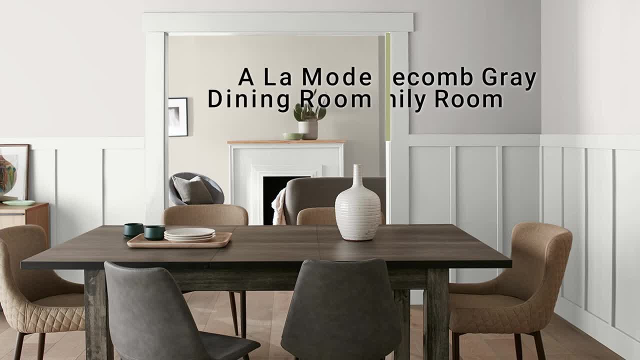 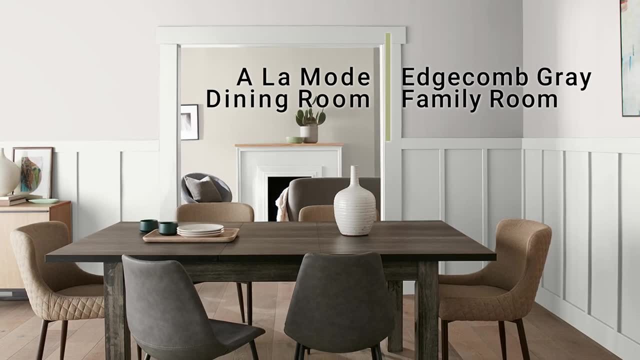 goes in pretty much the same way, And that's why I've used A La Mode. I like to use these colors in a yin-yang fashion, where maybe one room will have Edge Comb Gray walls with little bits of A La Mode influence in the form of accents, and then flip things in a nearby. 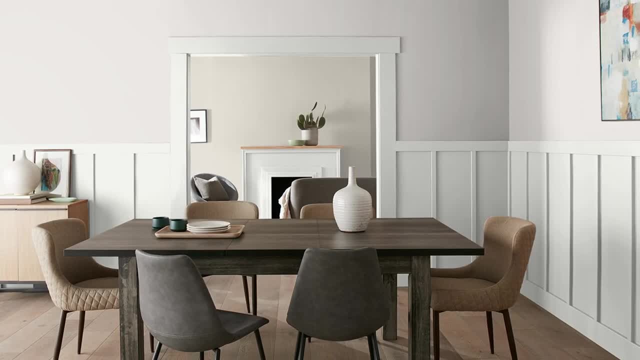 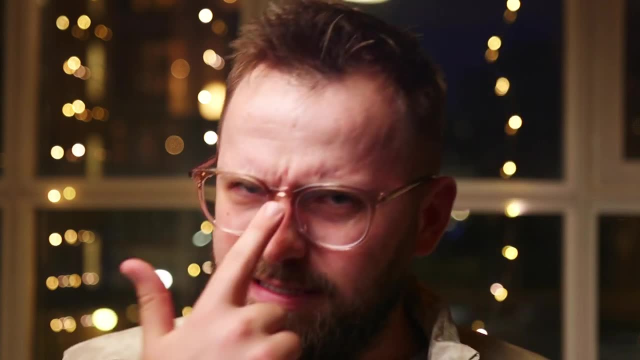 room with A La Mode on the walls and some more gold-leaning accents to cut through for a bit of a reciprocal relationship between spaces. James, this ain't math class. Get to the next color, you nerd. I know you just said that to me. Don't lie to me. We got our white. We got our light. 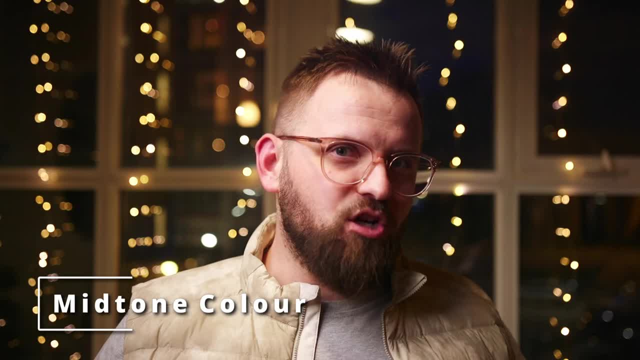 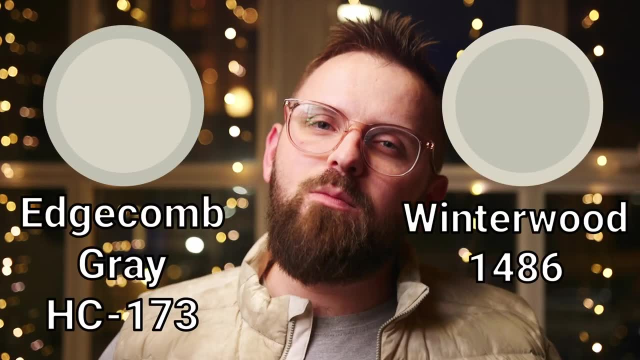 Let's go for a medium color choice. next, You may be tempted to pick Edge Comb Gray's neighbor, Revere Pewter, as the mid-tone color pairing, but that would be too easy. I prefer Winterwood from the Benjamin Moore Classics collection, which has a much clearer use of green mixed with gray and a touch of brown. 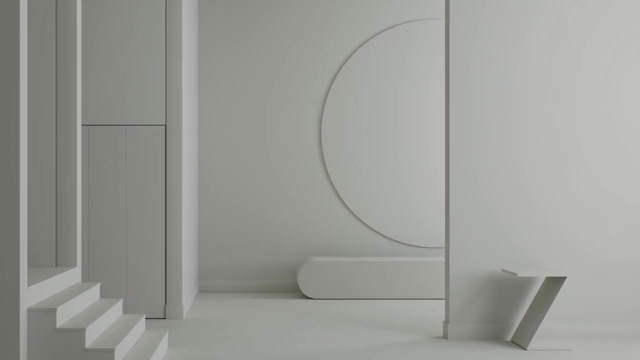 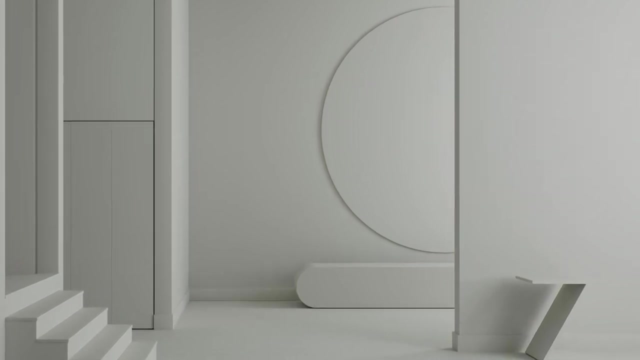 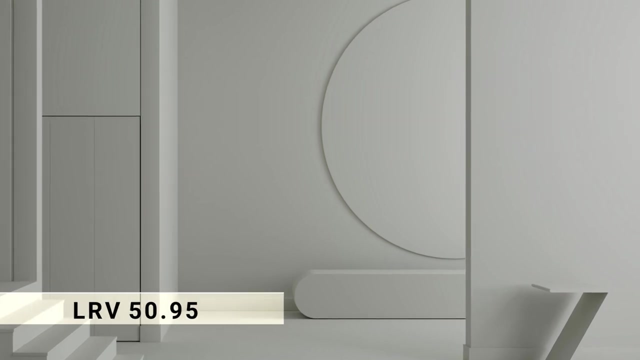 Almost feels like a fusion between sage green and taupe, which is absolutely perfect for a color like Edge Comb Gray. Winterwood will help enhance the beige aspect present in Edge Comb Gray, which is why I like using them together. They're also kind of right in the middle, darkness-wise, so it's not at a point where you can't use it on your walls. 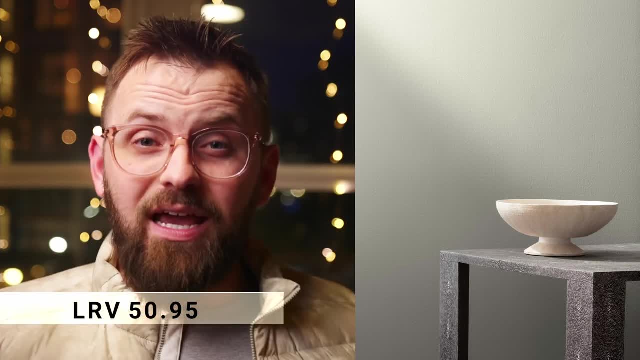 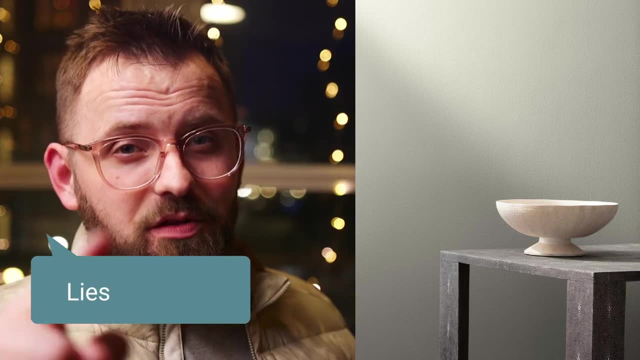 And this is especially the case in those rooms that get a ton of light. Winterwood is just going to be phenomenal on the walls and it really shines- no pun intended- with direct sunlight. So Winterwood and Edge Comb Gray, these colors are within that same wheelhouse, although Winterwood 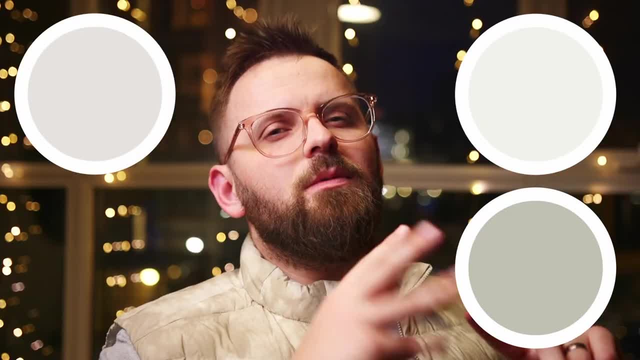 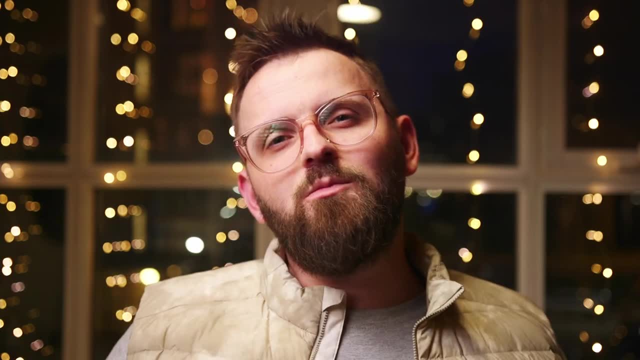 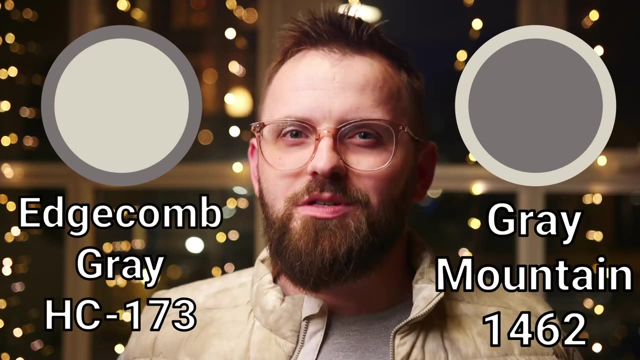 isn't quite as warm-feeling. Light, light, medium and now dark. The fourth color pairing, Because we found a partnership between Edge Comb, Gray and Winterwood. I wanted someone for my buddy Alamode, And that paint color is Gray Mountain. This is a stormy red undertone, taupe from the Benjamin Moore Classics. 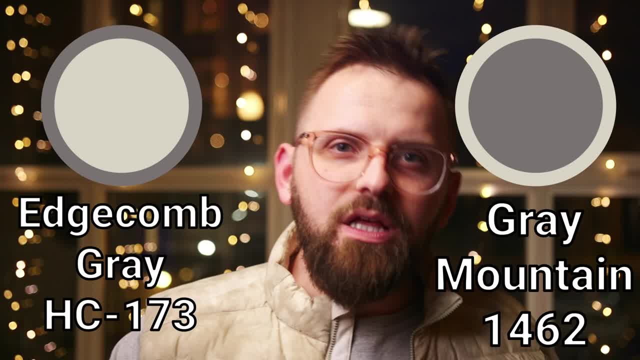 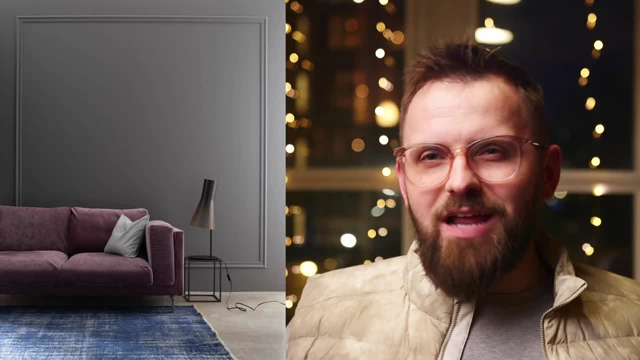 collection, color code 1462.. And it has a noticeable increase in depth from the other colors. Of course it does. It's the dark color pairing. It's got to be dark, right? What's fun here is Gray Mountain actually complements Winterwood and Edge Comb Gray, where the undertones are sort of 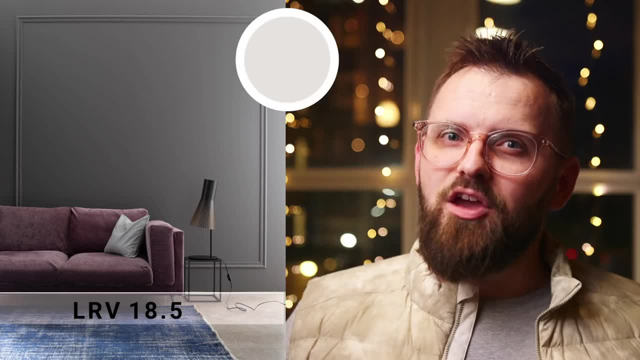 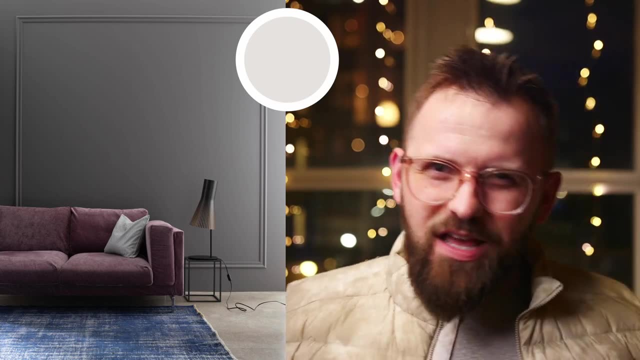 a dynamic look On the flip side. next to Alamode they almost kind of neutralize each other, Where the pink undertone in Alamode becomes softened next to Gray Mountain. So you can really have some fun piecing these colors together and coordinating them in whichever way you see fit, Whether you 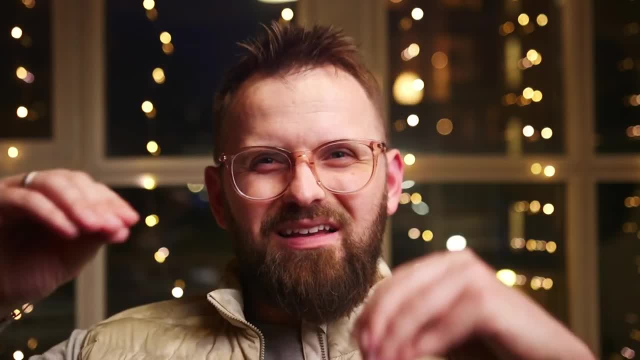 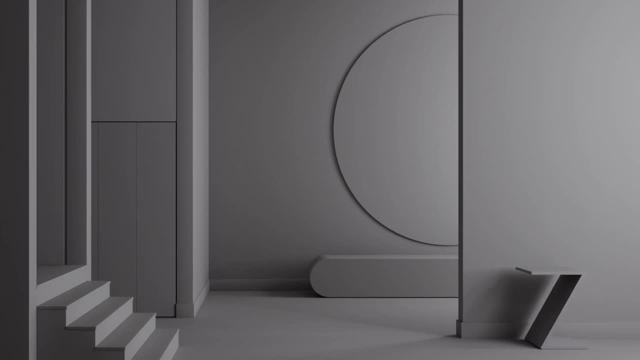 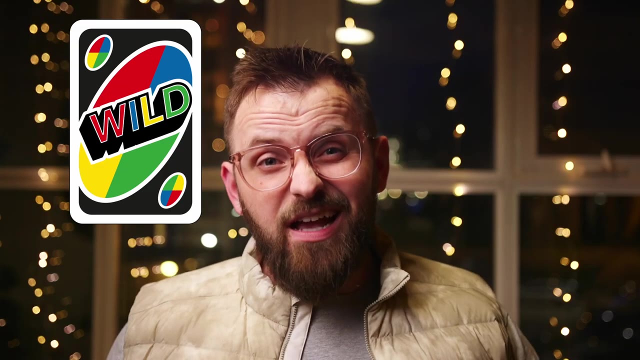 want them to coordinate or kind of complement and sort of clash in a good way. I will say that the red undertone in Gray Mountain can nearly disappear in certain lighting conditions and feel more like a stormy gray, But that's also what gives it its character. The final color to fit alongside Edge Comb Gray. 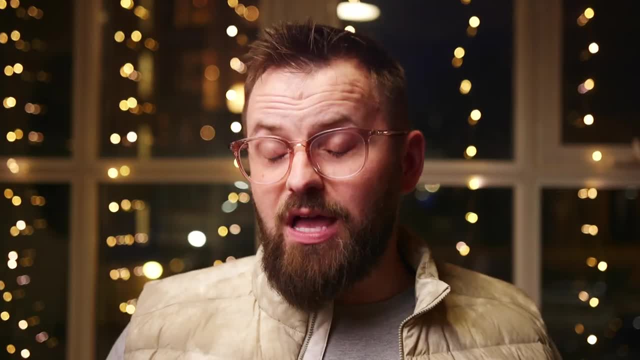 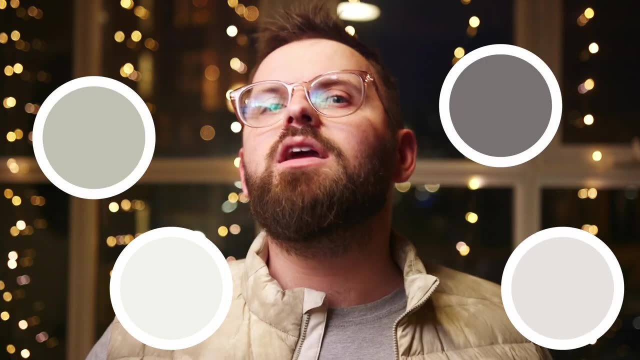 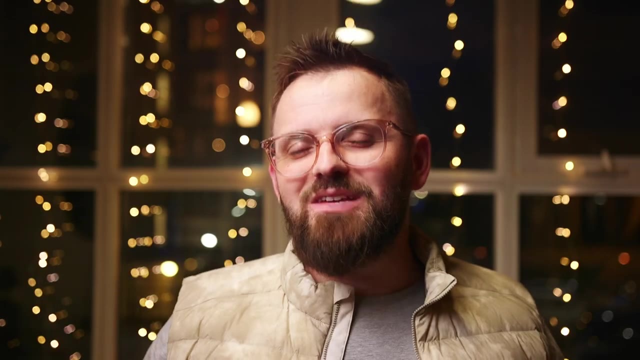 is our Wild card. So just a quick recap here We have our white in Oxford White, our light in Alamode, our medium in Winterwood, our dark in Gray Mountain and finally our daring color, which is a bit of an accent, I would say Another color from the Benjamin Moore Classics collection. It is 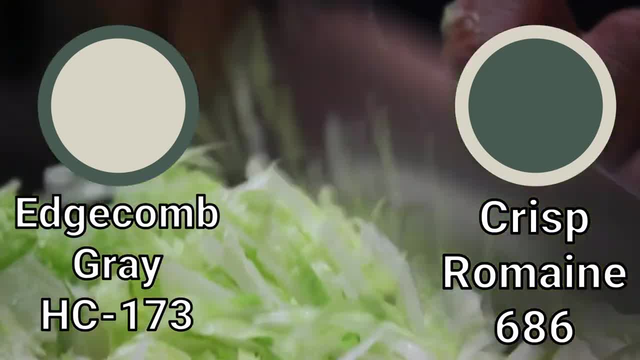 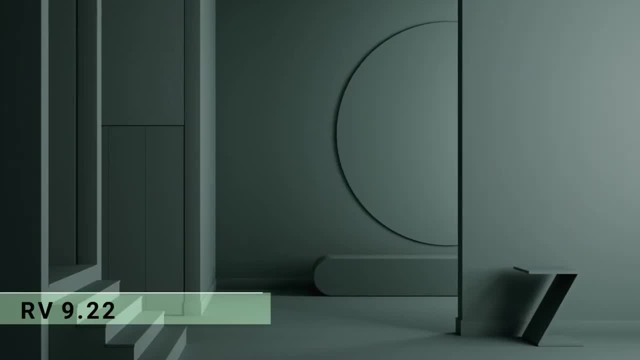 Crisp Romaine, which is a very dark shaded green that still possesses a slightly darker shade of green, And it's a very dark shade of green that still possesses a sliver of cozy warmth. You'll notice this entire color palette was free of any unapologetically blue. 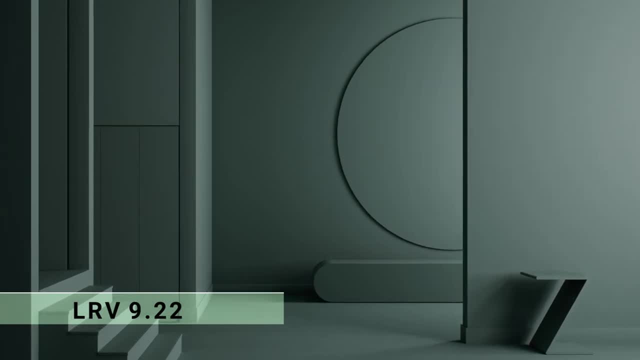 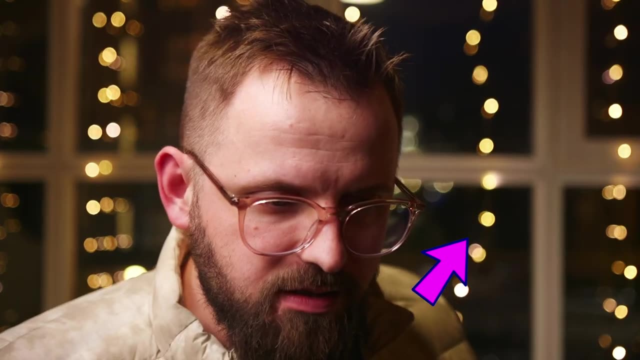 cool colors, So I wanted to continue that trend but also give you something that had a strong color hue to change things up There. a fast five color palette for Edge Comb Gray. I'll try and be faster next time.